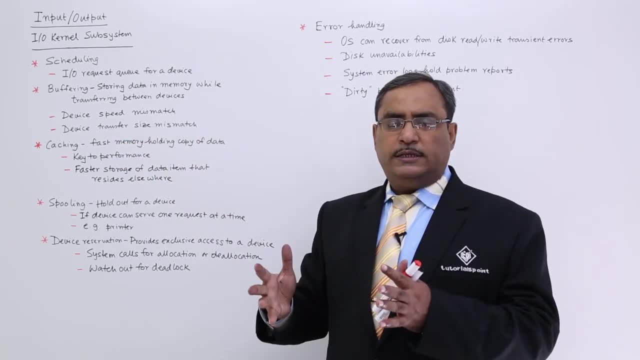 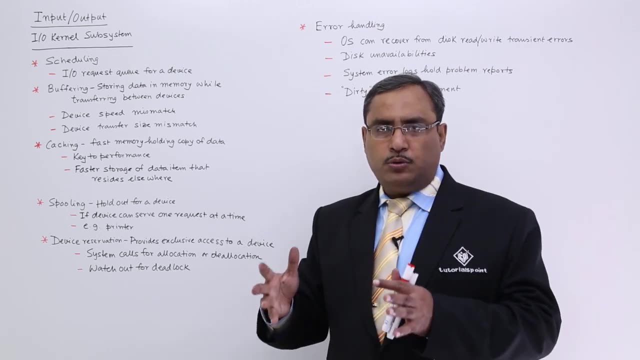 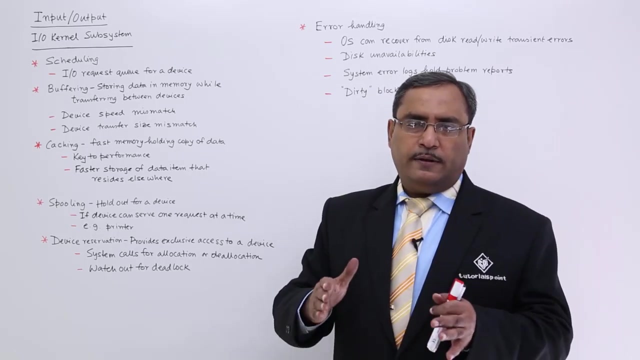 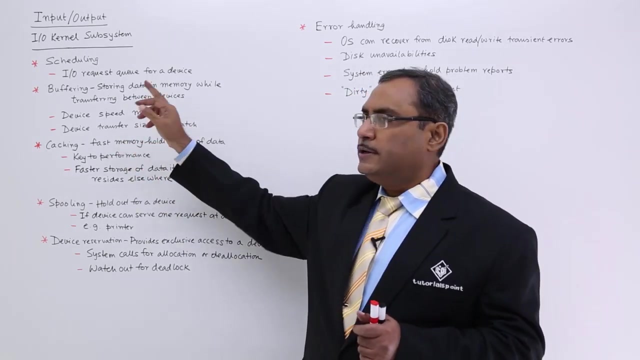 Device transfer size mismatch. So device is trying to put huge data but the DMA is not in the particular mode to accept that data In one shot. So in that case the buffer space will be utilized for transferring of huge amount of data. And here, in this case, the transfer size mismatch can be handled by the process known as the buffering. 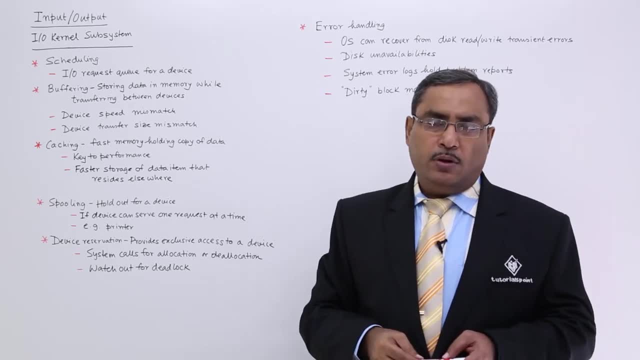 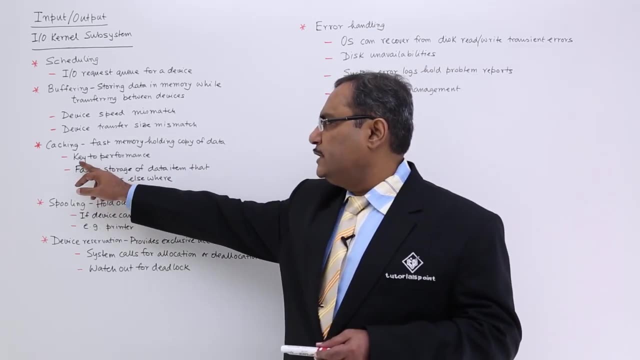 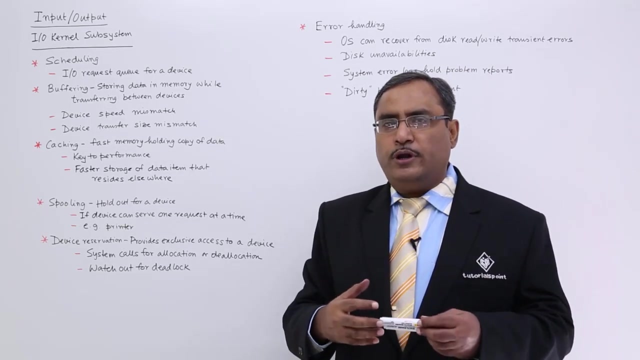 Caching, First memory holding the copy of the data. Obviously, that is the difference between the buffer and the cache. What is the difference? The difference here is that also, it is key to performance. If we have having the caching, caching caches have a is the fastest memory, external memory. so, as a result of 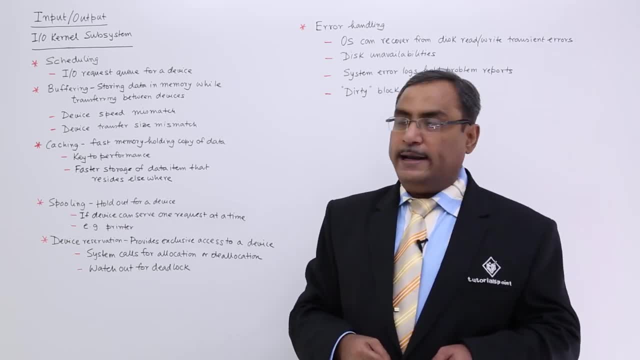 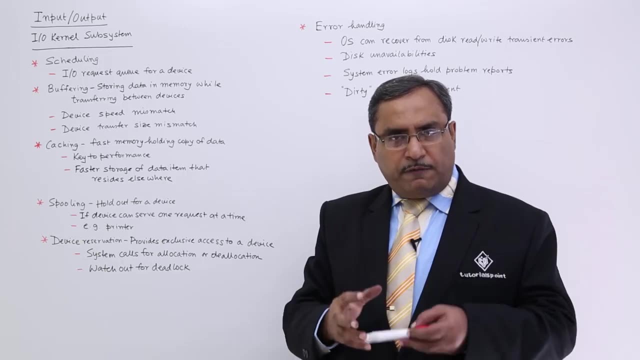 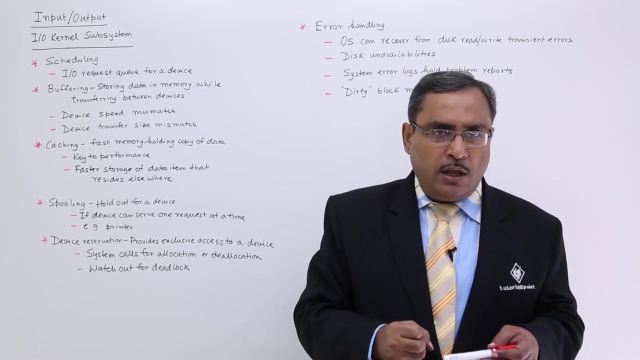 that the performance of that whole system will get enhanced. the faster storage of data item that resides elsewhere. that means the buffer is always holding that particular data which is now in transfer. but the cache may contain some other data which has been read from some elsewhere, some other. 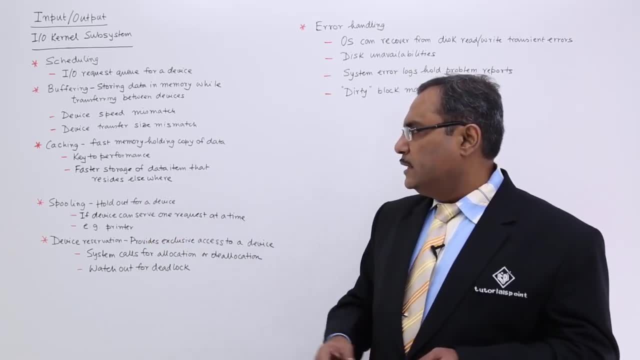 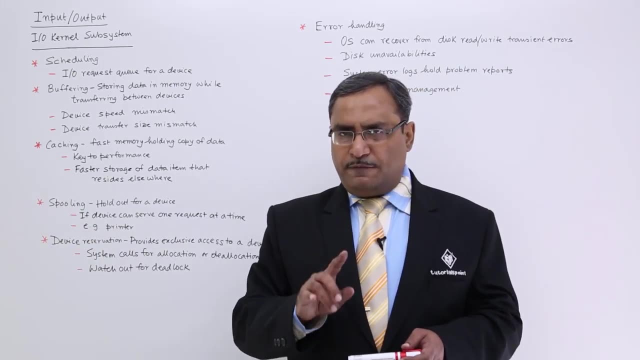 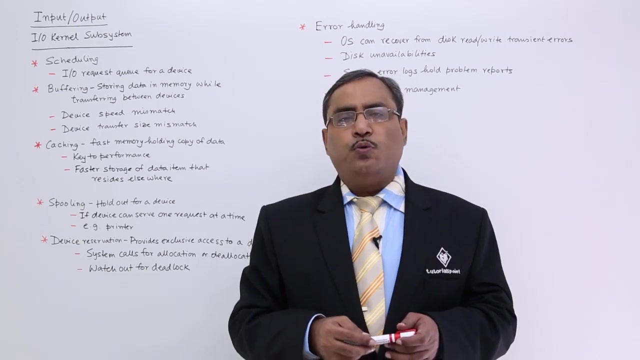 sources. spooling hold out for a device, the topic, the term is spool. s p w o l means simultaneous peripheral operation online, so that is the full form and in short, we usually call it as spooling. the spooling means what? let us suppose we. 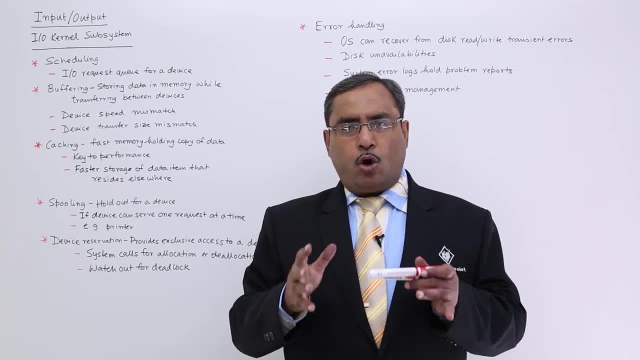 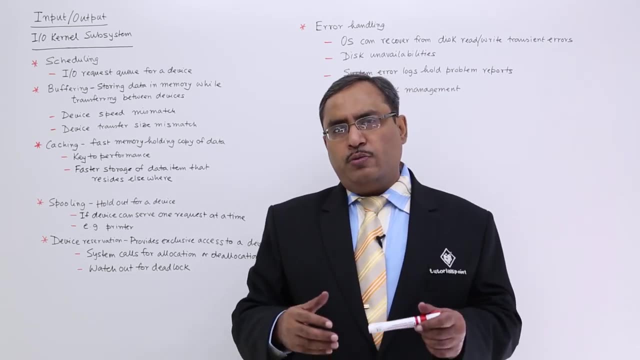 consider a printer. the printer can print a document one at a time. but if multiple documents have got requested to get printed through a computer, then the printer can print a document one at a time. but if multiple documents have got requested to get printed through a single printer, then what will happen? then all those processes will get. 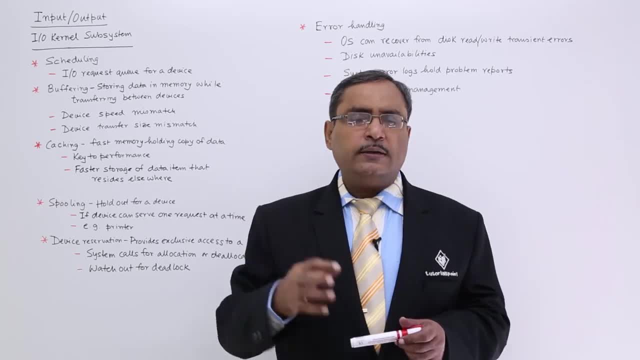 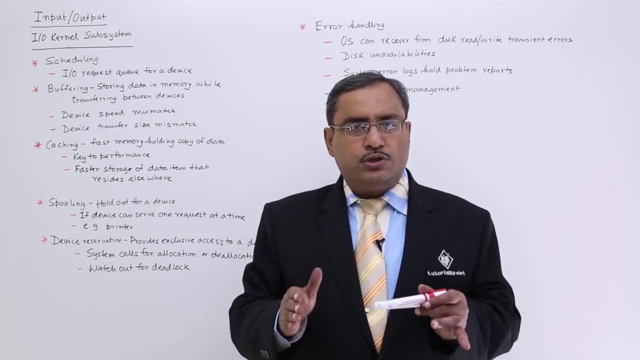 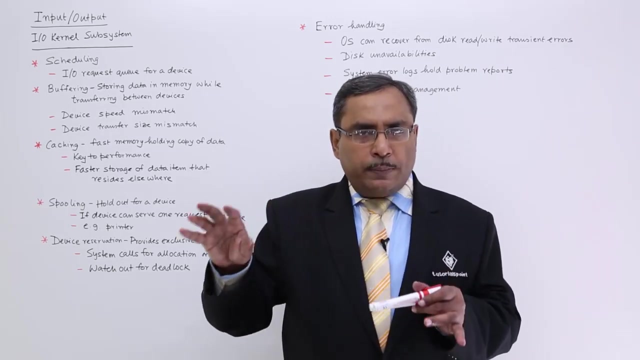 blocked until and unless the printer can print the respective document. so in that case, what will happen? there will be a separate hard disk space which will be used as a spool buffer, where all those documents will be kept in the print ready mode and whenever printer will get available, then from the spool buffer the 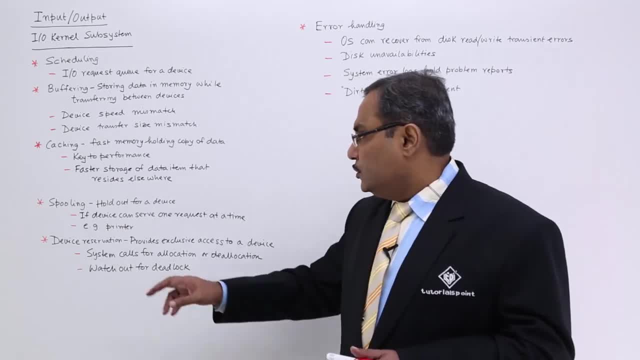 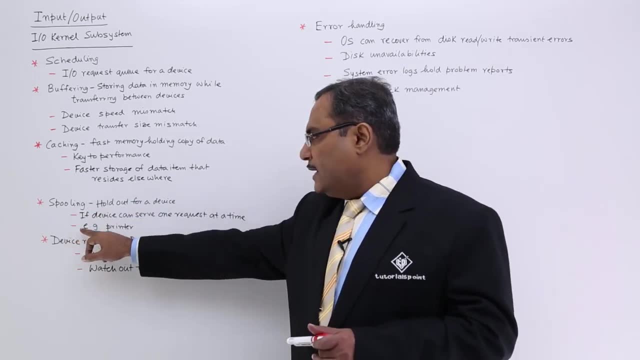 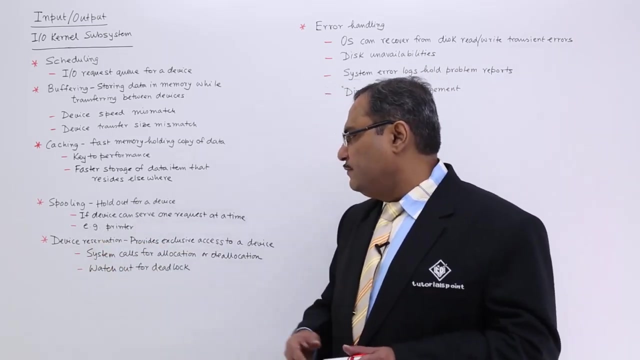 printing job can be initiated one after another, so it if device can serve one request at a time, then this particular spooling is required as example printer. also in my statement I use this printer as an example. device reservation provides exclusive access to a certain device, so 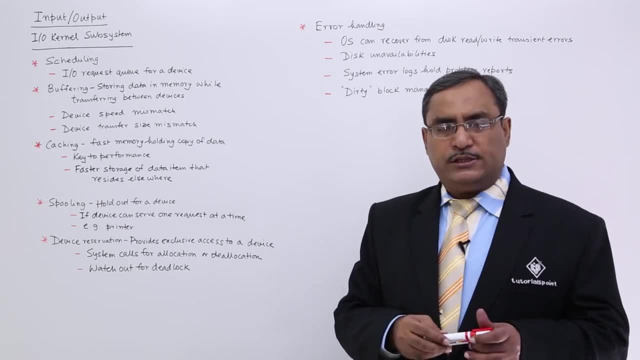 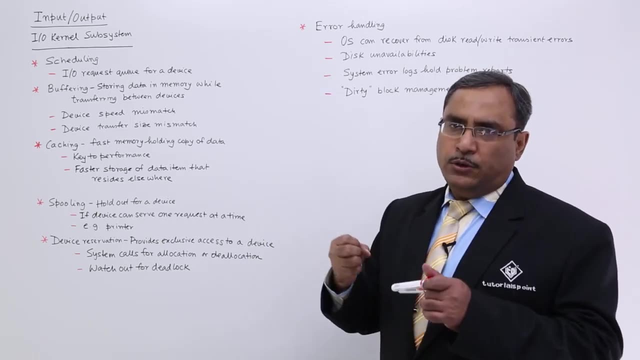 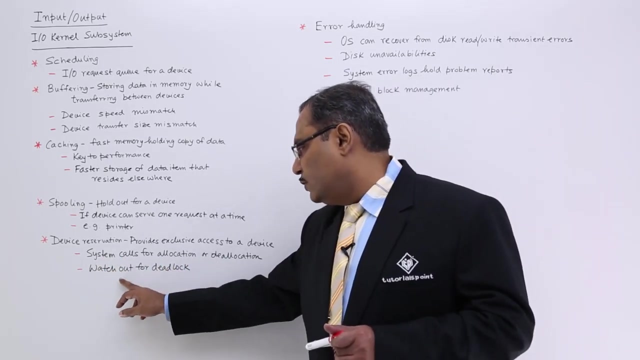 device reservation means, let us suppose, a particular device is to be used in a very dedicated way. so in that case this, that device reservation will help that That very device will be used only by that particular task. Systems calls for allocation or deallocation. watch out for the deadlock. 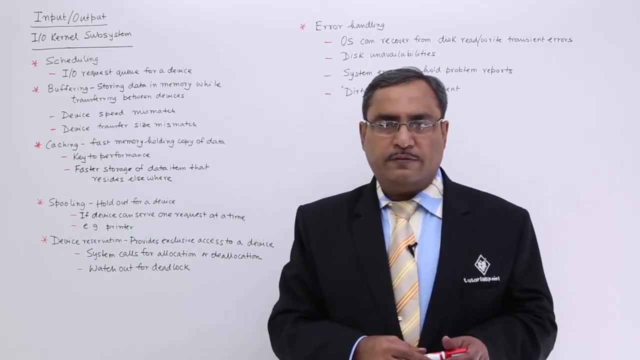 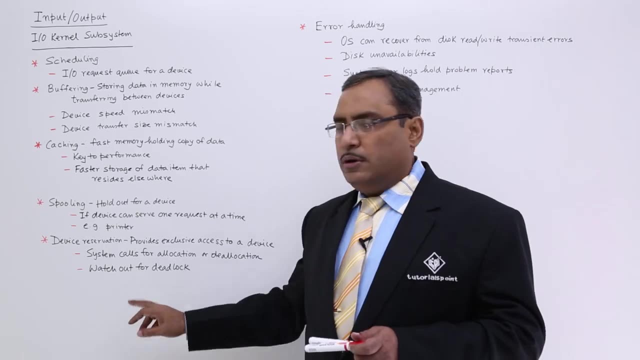 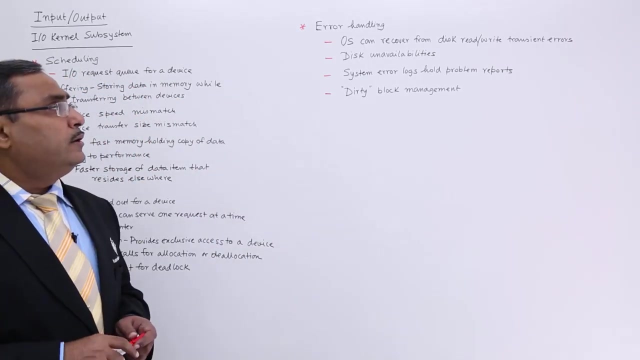 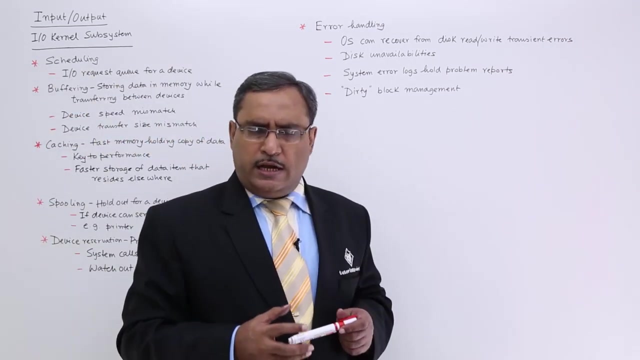 So these things will be required in the device reservation. Let us suppose a deadlock situation has occurred, So this device reservation can check and watch out whether any deadlock has occurred or deadlock is not there. Other points is error handling. OS can recover from disk, read, write transient errors while performing read or write operations. 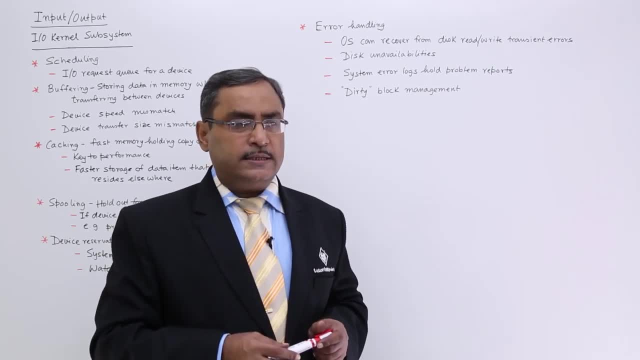 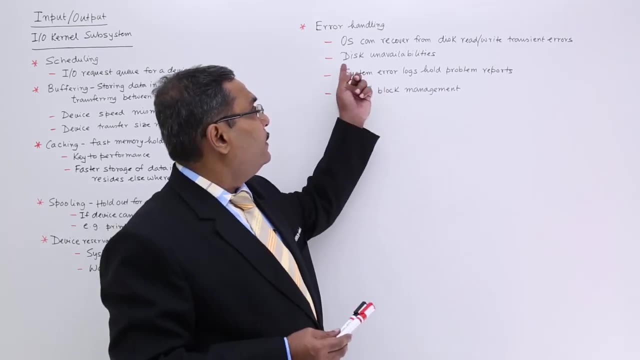 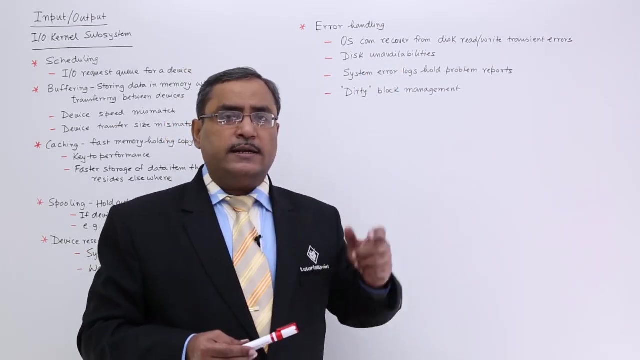 different kinds of errors may take place. So for the transient errors, this particular OS can recover from disk read write Also. the disk may be unavailable. the disk may be unavailable. So whenever we are performing the read write operation from a disk, some transient errors. 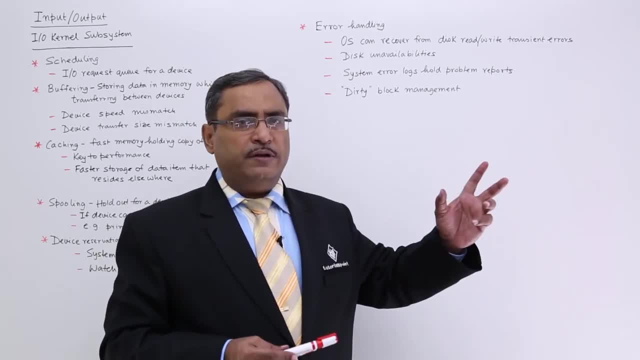 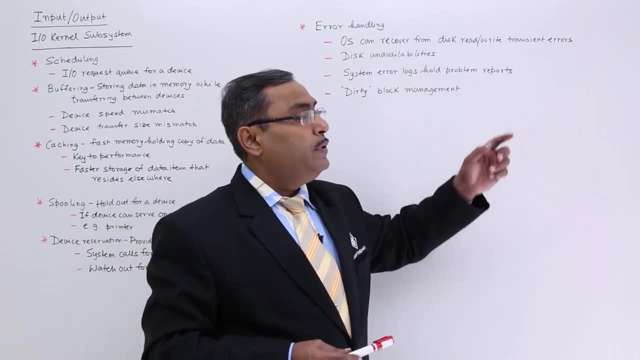 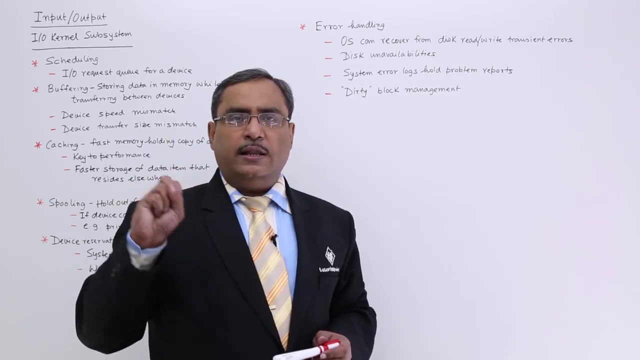 may take place, some unavailability of those devices may take place, And that will be handled in this error handling And system error logs hold problem reports. What about the problems we are facing? That will be logged on a certain database so that from there later we can generate the 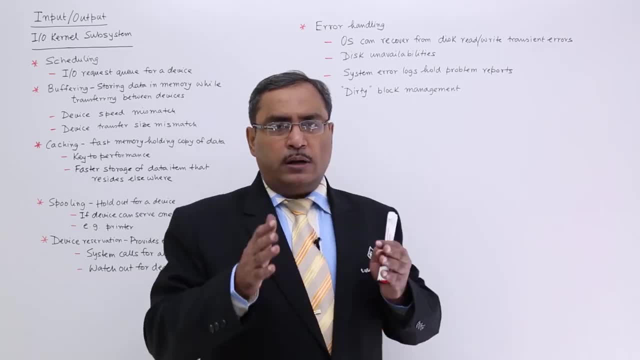 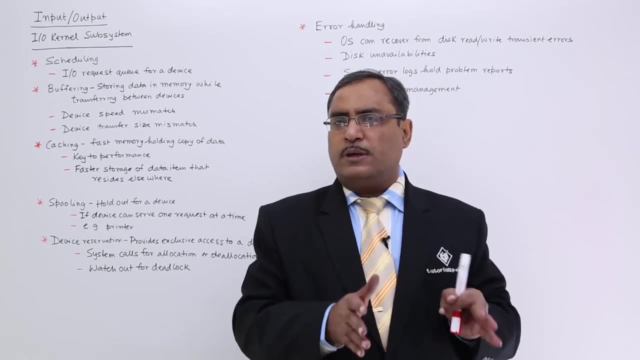 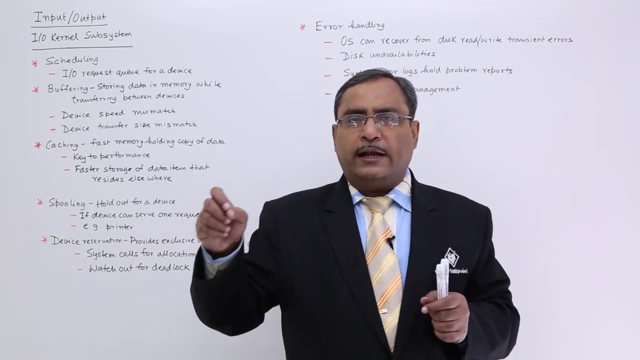 reports And dirty block management. let us suppose one block has been transferred from the secondary storage to the DMA buffer. In the meantime, somehow, due to some reason, the disk storage has got changed and that very block which is Now in the buffer, that content on the disk, has changed. 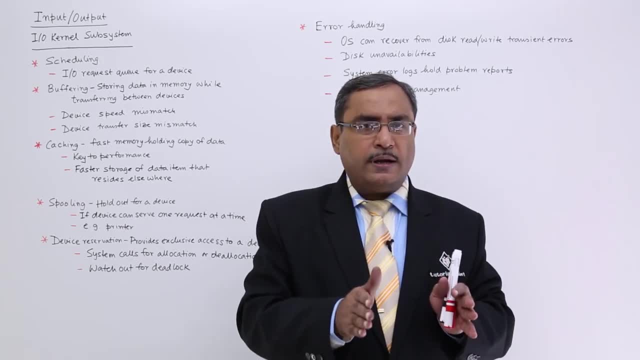 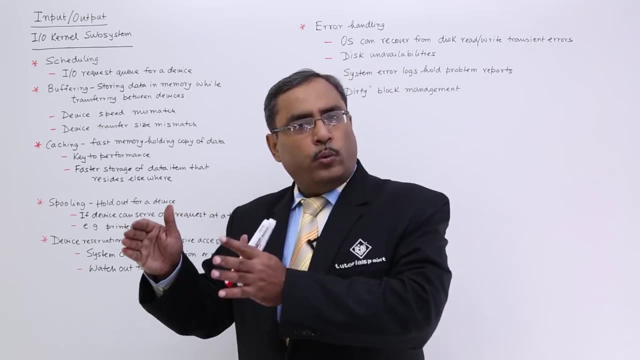 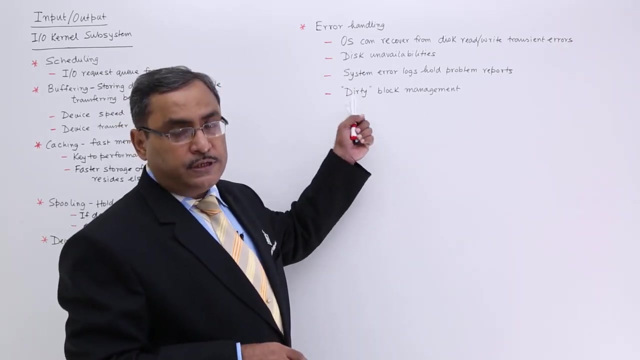 That means this particular block which is now in the DMA buffer is a dirty block. That means it is containing inconsistent data because the updated data which was there on the disk has got changed. So this dirty block management is one of the features of this error handling. 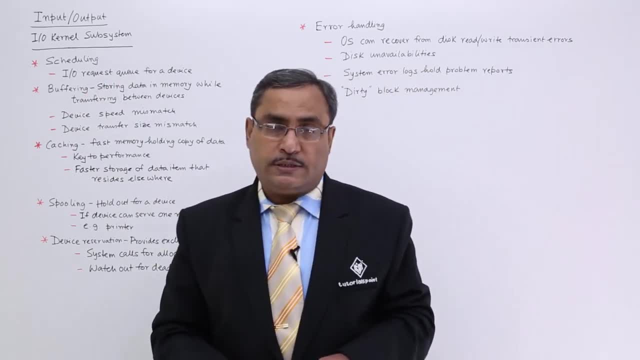 And each and everything will be done by this IO kernel subsystem. I think we have. 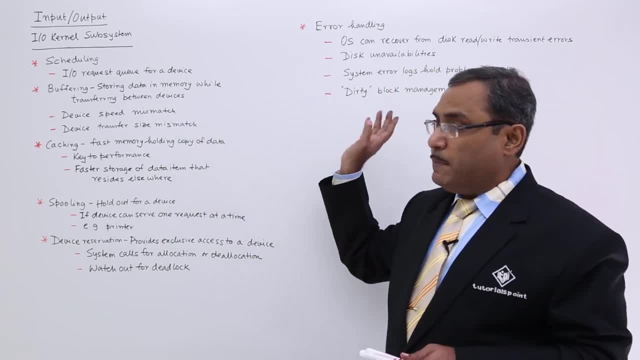 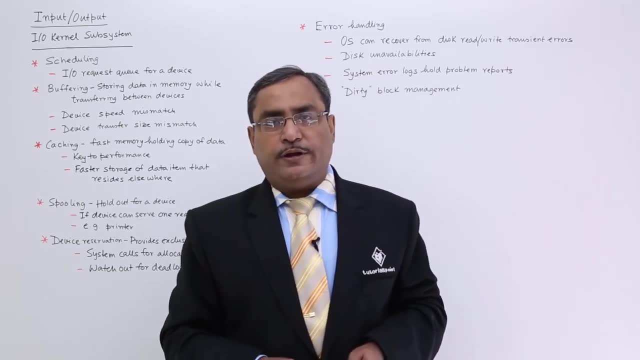